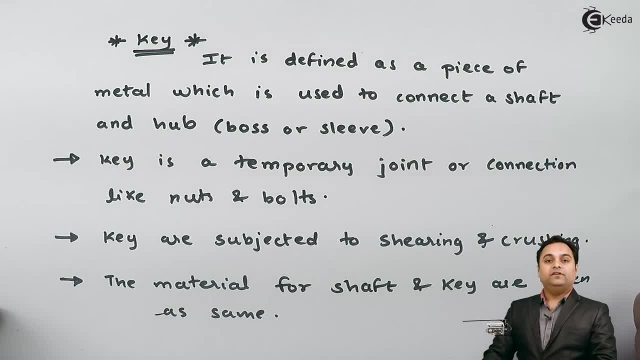 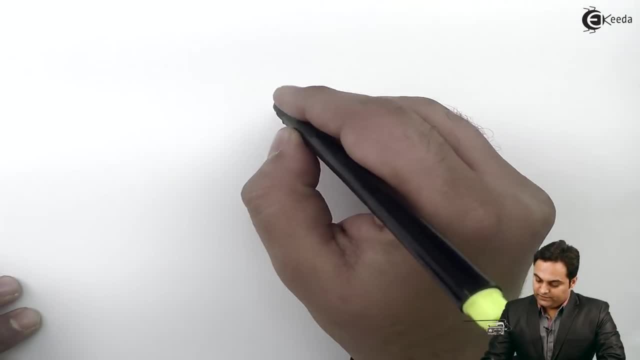 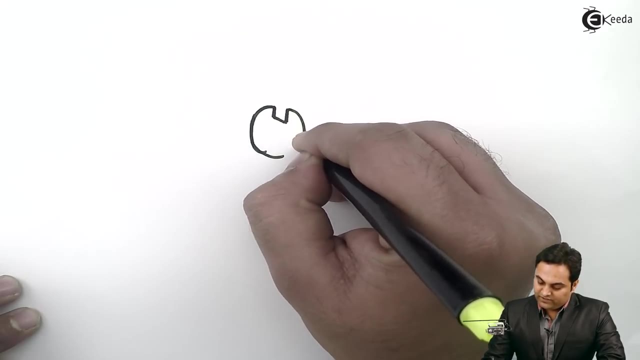 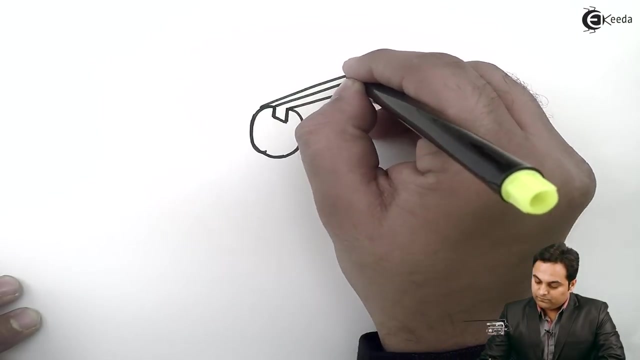 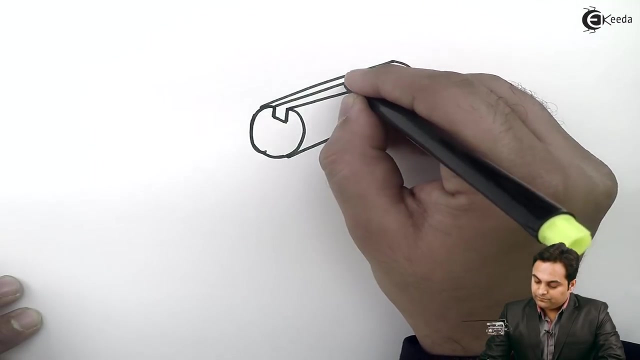 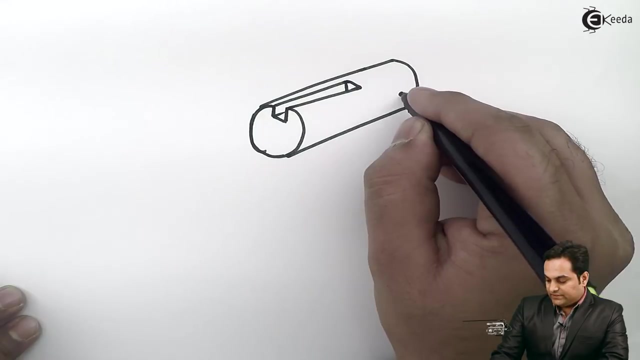 Now I will draw a diagram of a simple key and explain how it is used as a temporary connection For that purpose. So we've a shaft. Next, which is having is some value of its diameter. now that shaft will also have some length, like this: now, as we can see here, this is a shaft. next, here, some. 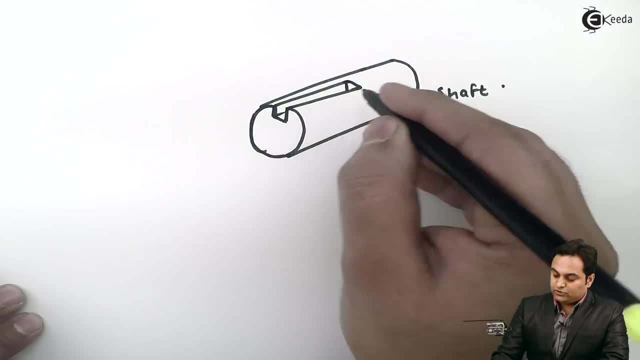 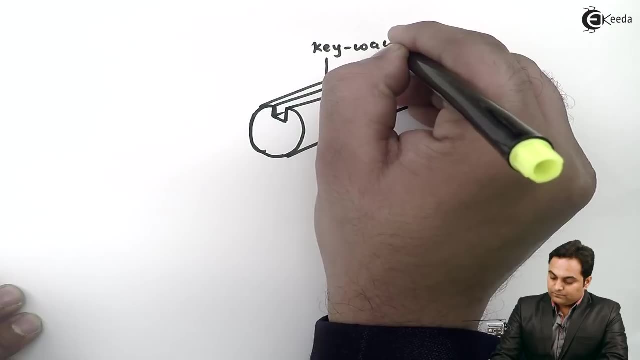 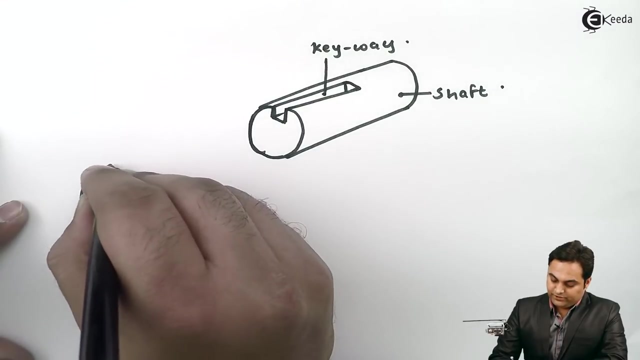 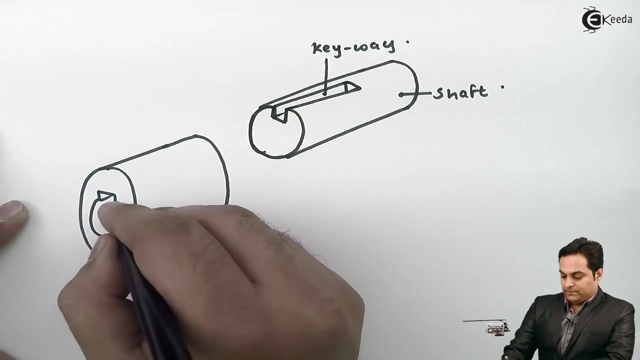 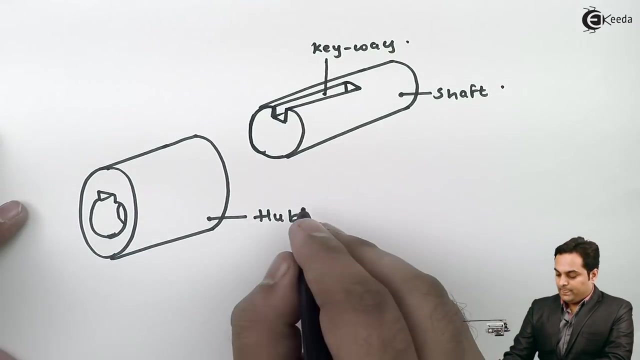 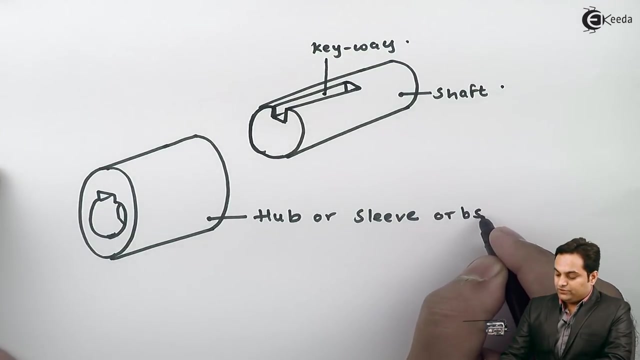 groove is made. this groove is called as key way. next here I am drawing another member which would be called as a hub. now this is either called as hub, or it is called as sleeve, or you can say it is also called as boss. now the key way is there in the shaft. a similar kind of 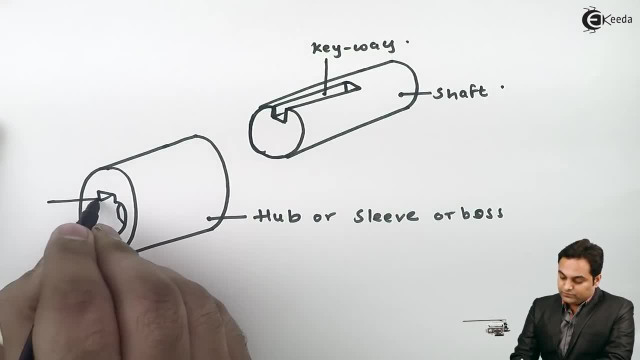 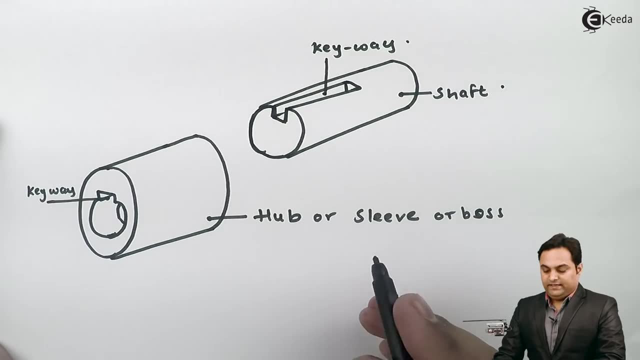 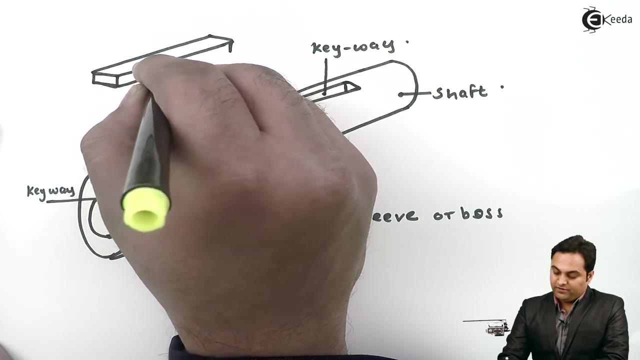 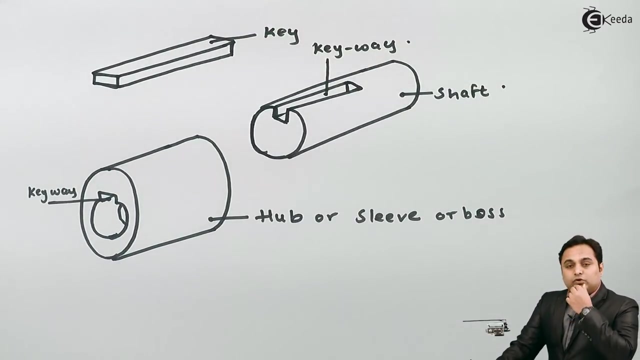 key way is also there in this boss. so here I can say that this is also a key way. next, here I am drawing this member and it is called as a key. so now how the connection takes place. see, if I want to connect this shaft and sleeve what I will. 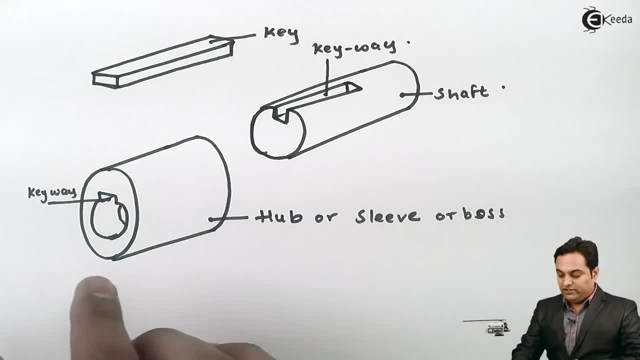 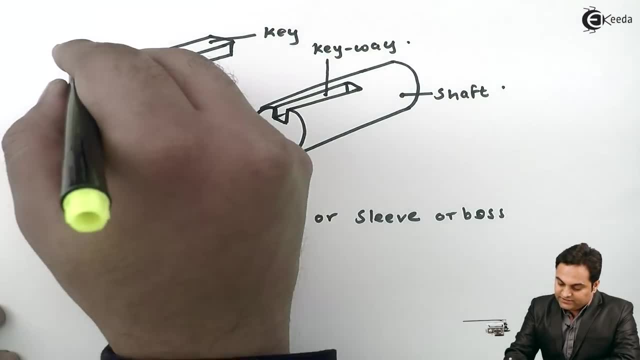 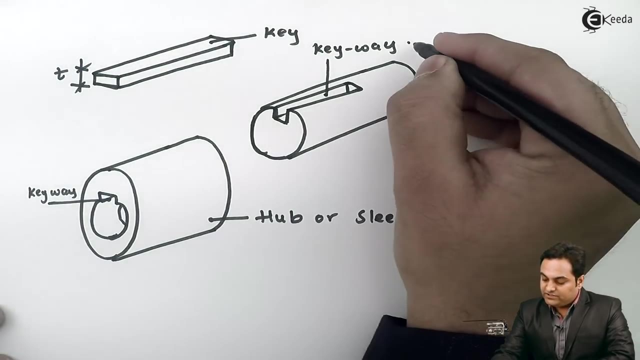 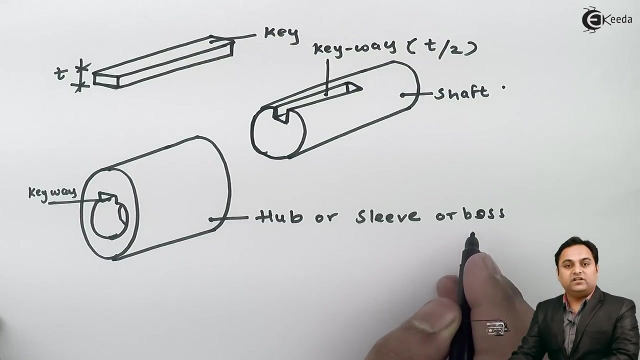 do? I will just put this shaft inside the hub next. So this key, I will say that its thickness is small, t. So half of the thickness, that is, this keyway has thickness as t by 2.. The keyway which is there in the sleeve, or boss, this also has thickness of t by 2..